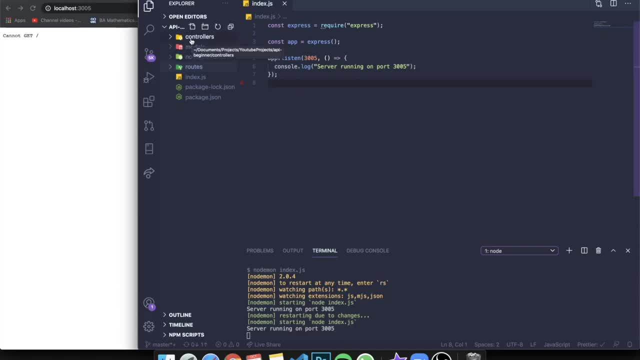 cool, But you can see here on the side that we actually created three different folders that didn't exist when we created this project. One of them is the routes folder, the other one is the models folder and the other one is the controllers folder. Well, the routes folder is pretty. 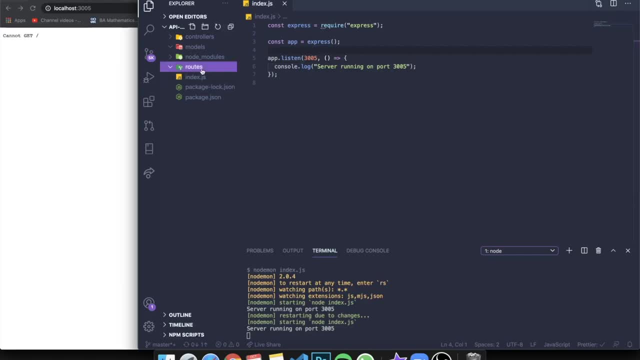 self-explanatory Routes is basically a folder where you include all of your different routes. So, for example, if I'm creating a project which has a user, so you would create a route called user and inside of there you would define all of the different stuff that you can do with a user. 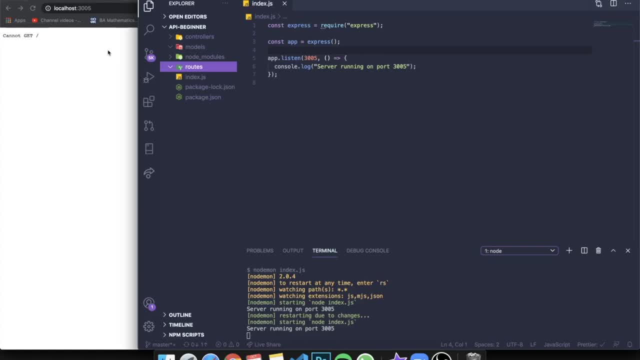 You can create a user, you can delete a user, you can update a user, you can do whatever you want with a user and everything you want to do with it, you insert it inside of that file. So the models folder, in contrast, is basically where you define the structure of your scheme. 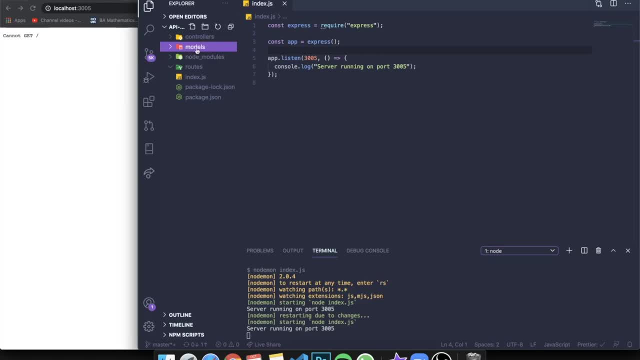 This explanation more simply, is basically where you define your database. So if you're using an SQL database or if you're using a NoSQL like MongoDB, it doesn't really matter. You will define it over here in models. Basically, I would recommend most projects use an ORM And in ORM. 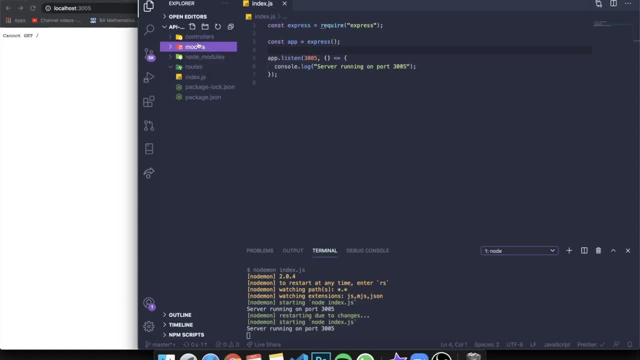 I had several videos talking about it. If you're using SQL, you can use SQLize. If you're using MongoDB, you can use Mongoose, But basically it's just a way to define your database. So if you're going to organize your queries in a way so that you're using normal JavaScript and treating them, 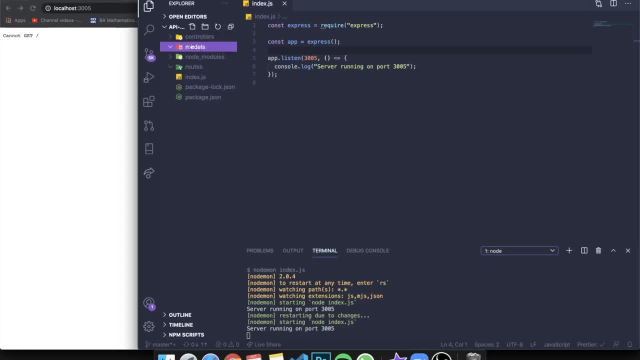 as objects. So basically, here is where you would define those models and you will define the database tables and everything inside of models, And then control is basically where you execute all of the different things you want to do with the data And it's basically where you construct. 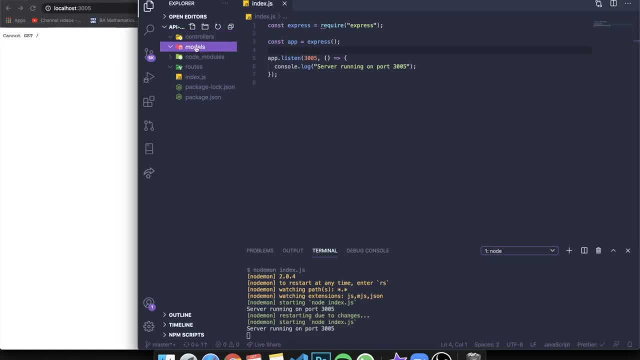 you manage the data, So you make the request to whatever database you create on the models and you treat that data. This might not make so much sense right now but as I keep working on a project, you guys will see basically the idea of it. So let's create a simple route And let's come here. Let's pretend like 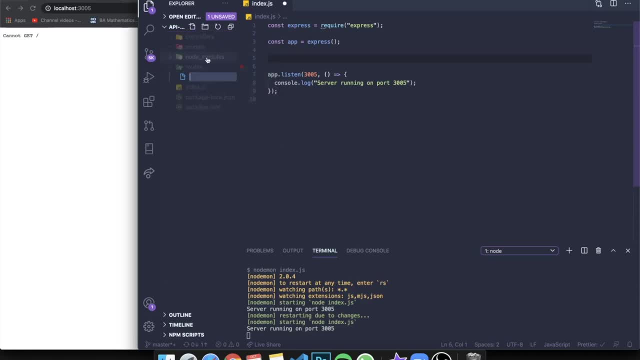 we're creating a project where we need to work with a user. So in the routes folder let's create a userjs And over here we can just call an express variable and require express And normally when you create a route you can just come here. 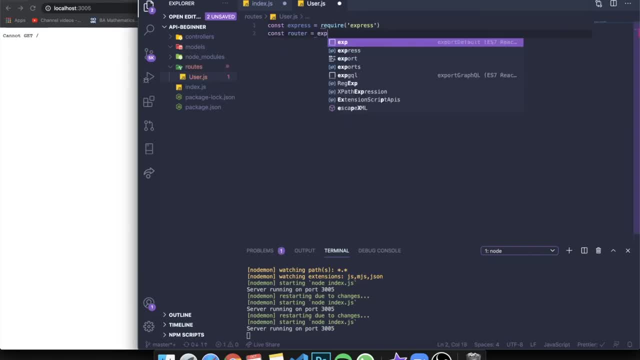 And say router equals to expressrouter. Okay, created an instance of a router And now we can use this router to make requests, Like, for example, if you wanted to make a post request, we could just do this. But, as usual, this is what I want to make, what I want to emphasize Basically. 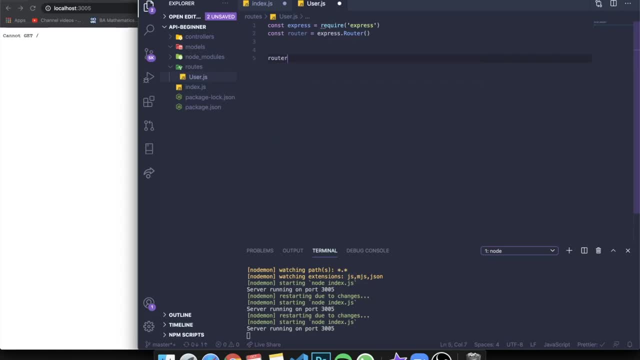 if you want to make a post request to create a user, you would usually write it like this: router dot post. then you would create a slash. I don't know Actually, just just create a slash, because we're going to come here to our indexjs And let's 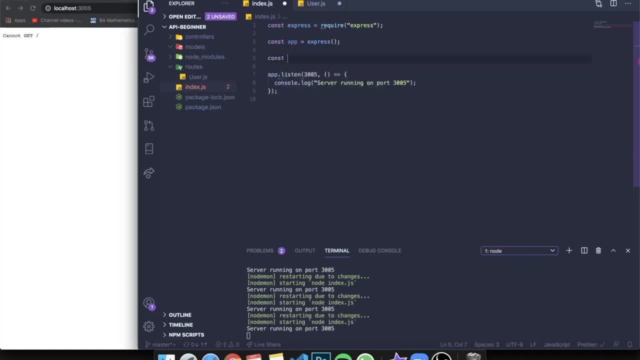 initiate the route, So const user routes equals to require. Then let's try to access the routes folder, So slash user. Now we have, we collected that, we have in our in our variable, the user route And then we can just write app dot use. 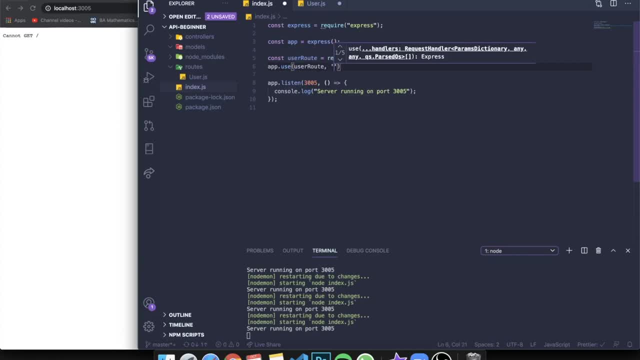 A user route And we can add the user route. Basically this is just saying, if you don't know what, how to use routes. basically this is saying that whatever is written over here is basically going to be accessible through this localhost 2005 slash user. So if we just say, app router. 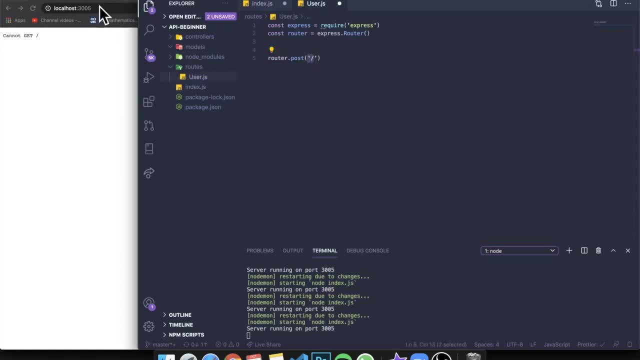 dot post slash. we're basically making a post request to the localhost 2005 slash user, So that should be fine. And then usually we will write rack and res to make a request and a response, And instead of here we'll do something like res dot send. You just created a user, something. 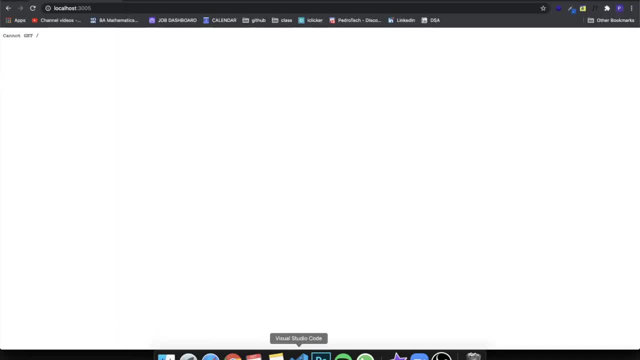 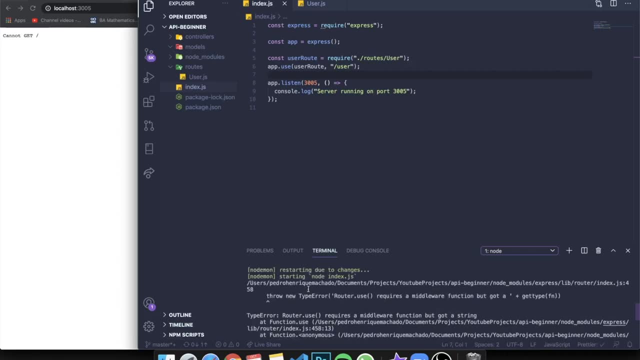 like this: Let's test this to see if it's working. So, for example, wait, what happened? My app crashed. a router is a middle of middleware function. What happened? Okay, oh, I guess I know what it means. What happens? So if you go here to the indexjs, I guess this: 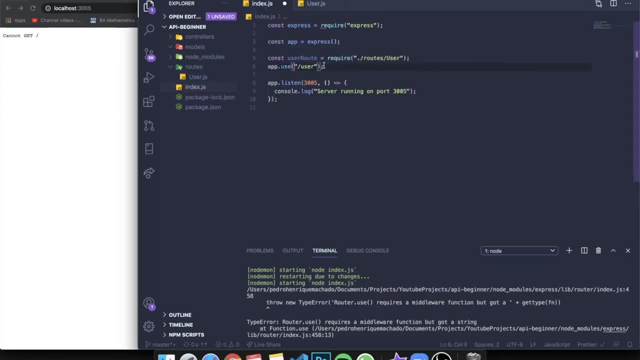 is the problem. We have to actually pass this first And then we pass the router. So when we save this, you can see now that the error continues. So I'm going to take a look at what happened And I'll come back. Okay, guys, I'm back. 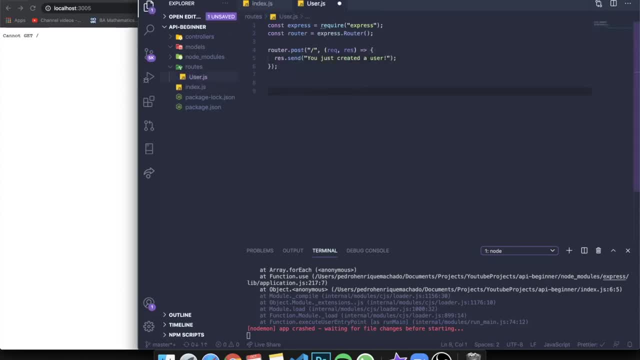 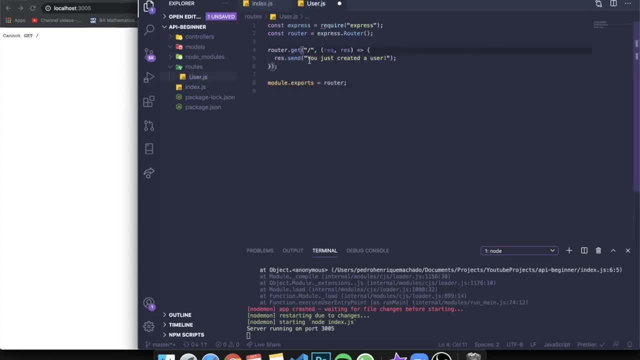 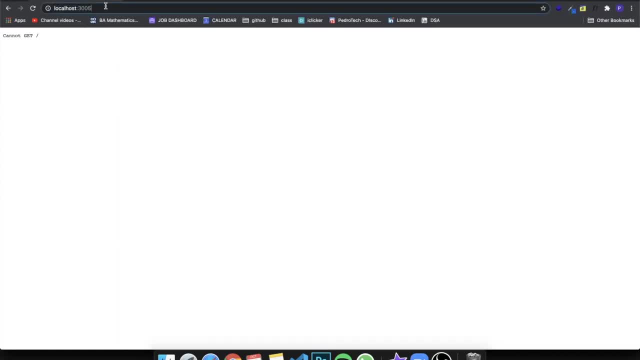 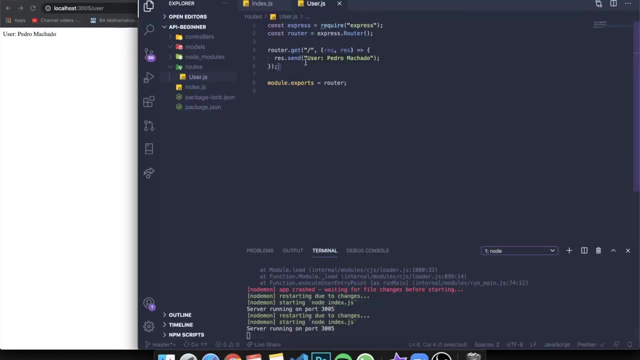 is my name. Okay, so basically, when we try to reach the slash user, you can see that it displays user Pedro Machado, But this isn't falling and VC. the reason why it isn't following is because we're working through, we're making the, the HTTP request, all. 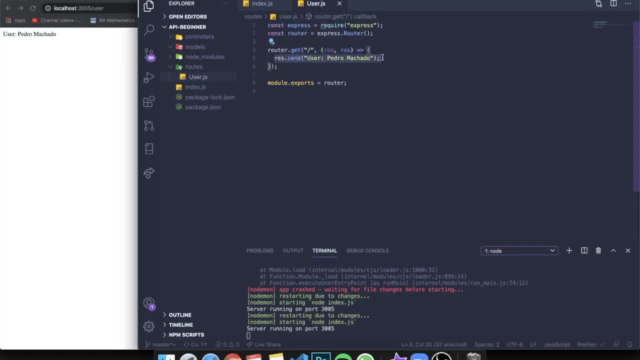 here we're making the the get request and we're working with whatever data we have inside of here. so basically, what we would do is we would make the query uh inside of the models and would receive the data from our database if we wanted to receive a user, and over here we would actually make a. 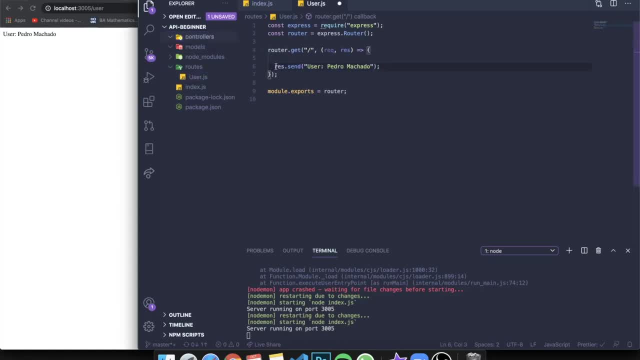 request to our controllers, and this right here would be all logic that exists inside of the controllers. so let's create a controller so you guys understand. i would come here and write user controllerjs over here and the user controller would actually be very intuitive inside of here. 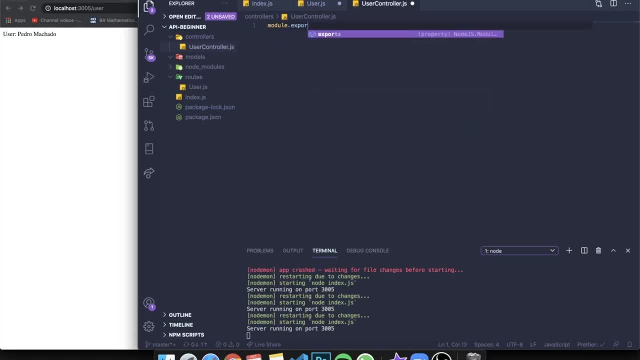 it would be basically a moduleexports and we would export an object and basically this object would contain all the different posts and the different http requests that we would make with regards to the user. so, for example, if we wanted to make a function that would relate to a get request. 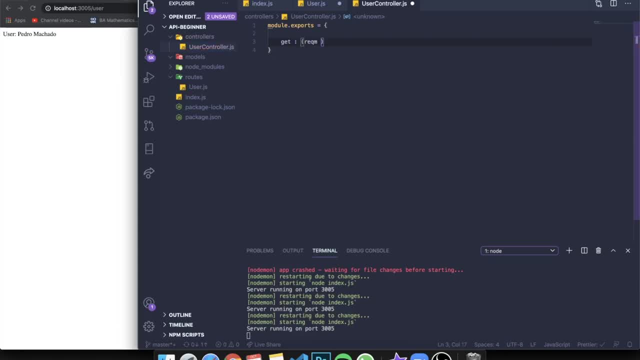 we could write get, then rec, rec, res and pass a function and inside of here let's paste the ressend. so this is where we define. whenever we want to make a user a get request in relation to the user, we would basically define it over here. currently we only have the get, but let's use this over here in our favor. well, 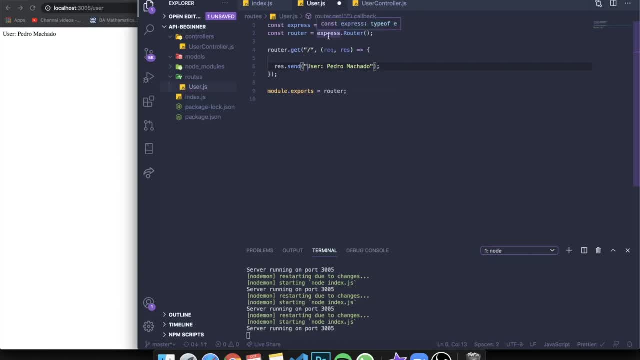 since we just created the user controller, we have to import the user controller. so let's first come here and write: get controllerjs over here. we have to import the user controller, so let's first come here and write: const controller equals to require two dots slash controllers. 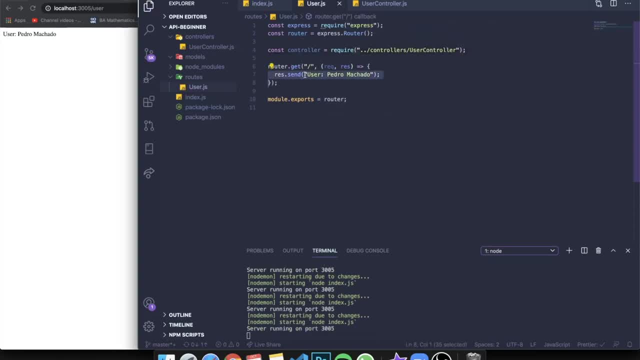 user controller. and now, instead of just writing ressend, instead of actually writing any function after the get request, we could simply pass that logic to the controller and come here and say controllerget. and now this knows that whenever we try to reach a get request, we can do that if we go to those other functions of the get request. and I'm going to ال Depoisки長, pathakinned Jean- get request. 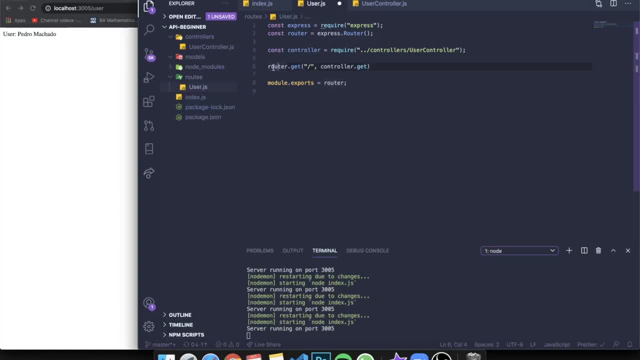 controllerget. and now this knows that whenever we try to reach a get request or you have an Imperial intitti, play scrum domingo and we frustrationally write true get request, you don't need to stop working with those functions. you can leave them. search for get request. wed nexttrackor zur Monger and on 안上の. 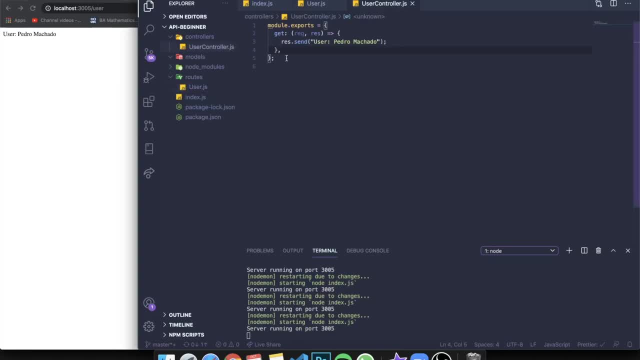 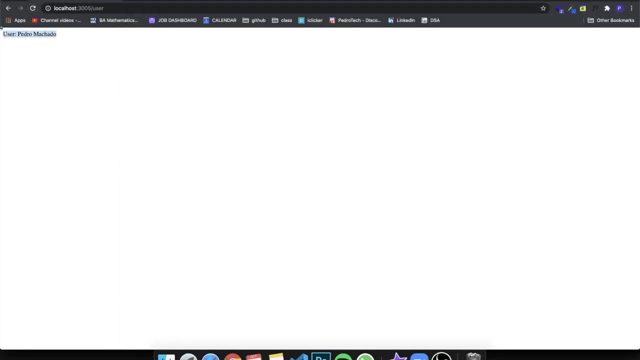 request for the user, it will try to go to the controller and it would see what a get request means. this is basically a way to structure. remember that it doesn't make any difference. the only difference is that you're following a very well known and very organized design pattern where you can just make. 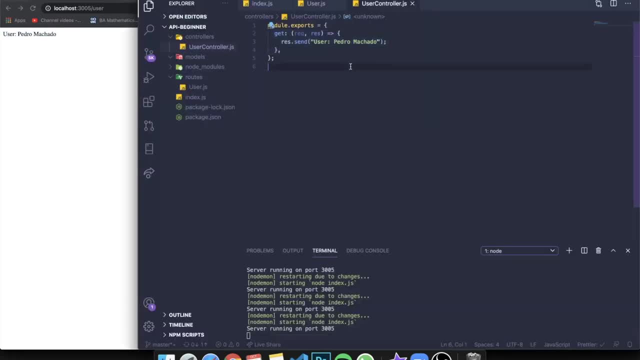 this make the project look a lot nicer and a lot easier to debug if you're trying to work with it, because you know that all the logic is separated into controllers and all the queries are separated into the models and all the requests are separated into the routes, and if you also have views in your 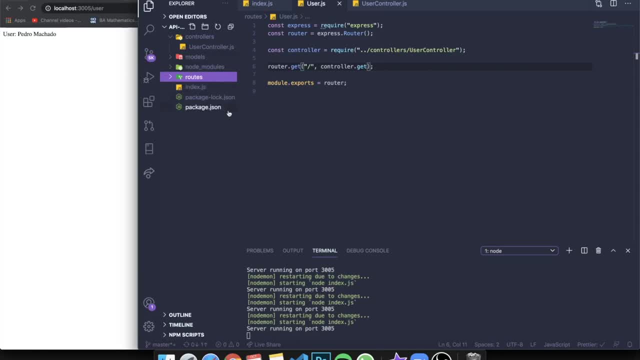 project. you would also know that your views are in a views folder. so this is basically the video. I hope you guys got the the gist of it. basically, you you would create, for example, a router dot post here and you would add the logic for the post on the user controller, if you wanted to make a putt. 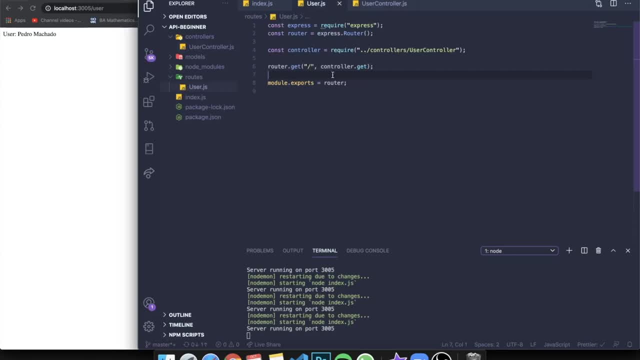 you would do the same thing. basically, I didn't want to make this video very long. this is basic, the basic idea of working with an MVC pattern on a express and no jazz project. so if you're have any doubts, please leave a comment down below. I would be very happy to. 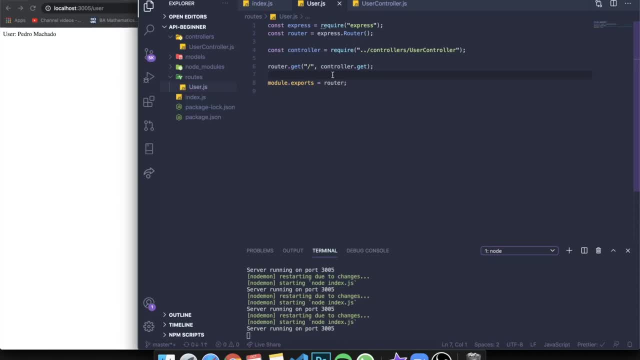 answer. I'm posting every single day, so if you would like, if you could please subscribe and leave a like down below, because I would really appreciate it. I'm also selling some merch, so if you would like to, to buy something it's like related to programming, coding, the it's basically. the link is down below it's. 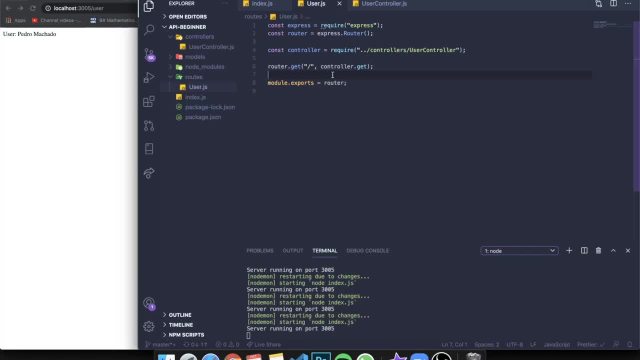 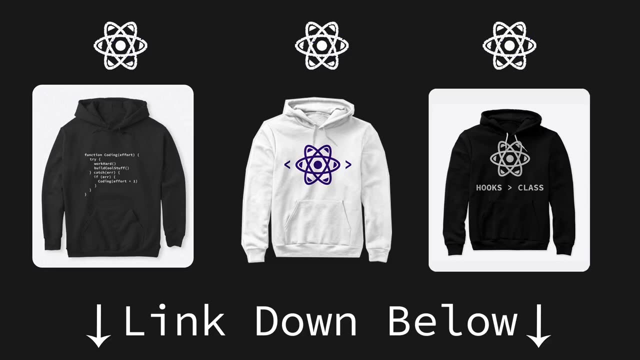 there. I think they're really cool. but also, if you want to see more videos, please leave a comment down below seeing which videos you want to see, and I hope you guys enjoyed it and I see you guys next time you.